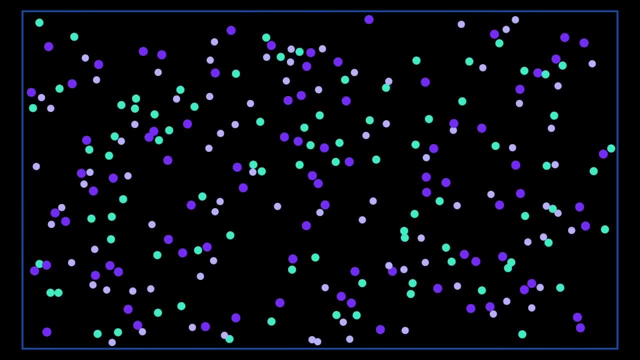 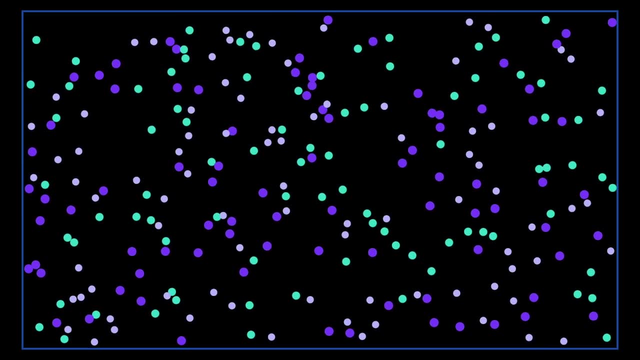 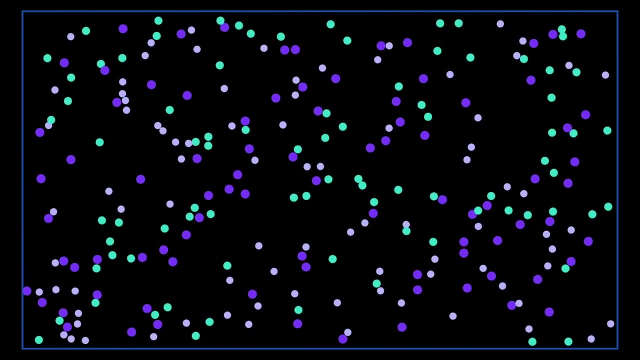 This right here is a simulation of 250 particles in an enclosed space. By the end of this video you have a good idea of how to create something like this. But the way I see it, this video is actually more than that. Physics-based simulations are a nice playground of sorts to explore a variety of interesting 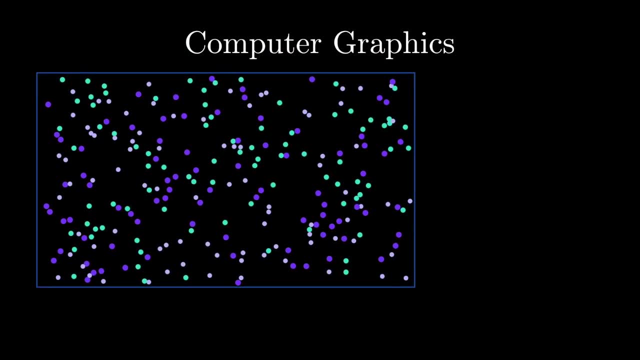 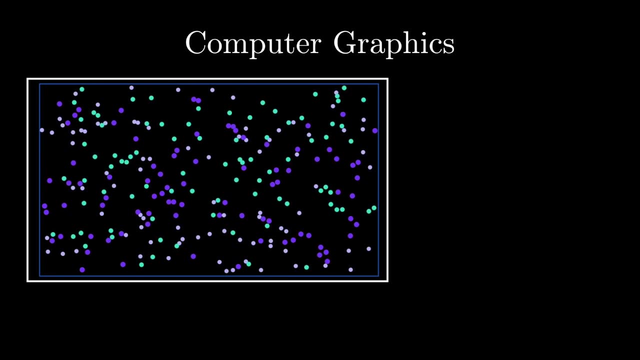 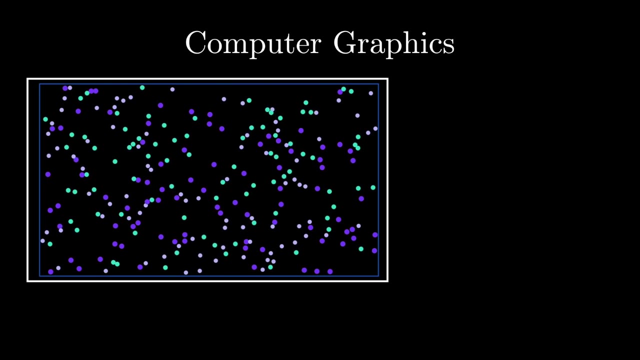 ideas in a field of computer science called computer graphics. In the process of learning how to build these simulations, we will encounter a lot of problems, and the tools that we will use to solve these problems show up all the time in computer graphics. So here's the plan for the video Before we understand simulations. 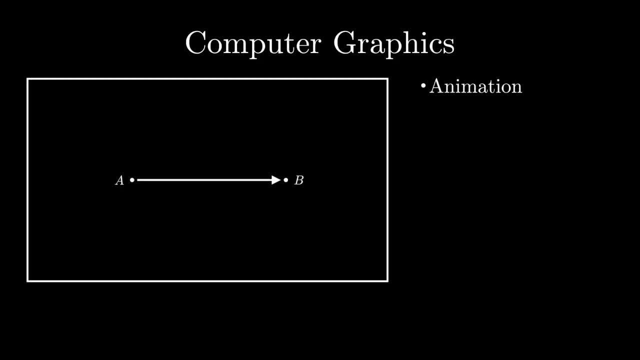 we'll take a look at some of the core principles of animation from a computer graphics perspective. With this framework, we will then build our first simulation, which will introduce a variety of ideas in particle dynamics, collision detection and collision responses. The last half of this video will then be dedicated to managing the complexity of 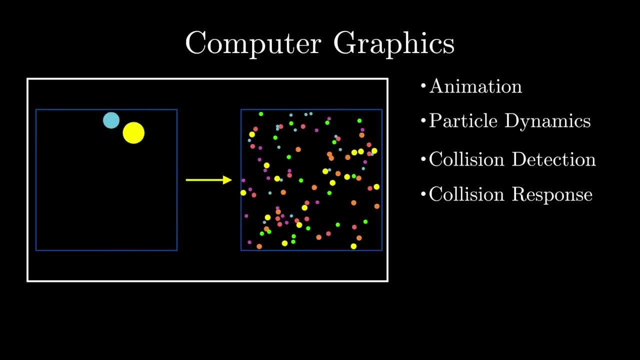 larger-scale simulations. This will be the first part of the video where we will take a look at some of the core principles of animation. Not surprisingly, the more particles you add, the harder it is to make accurate simulations in an efficient manner. This. 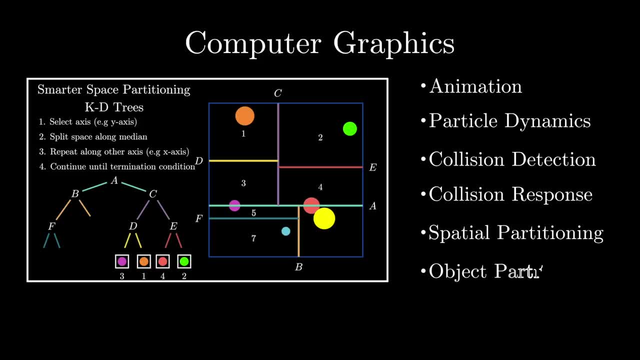 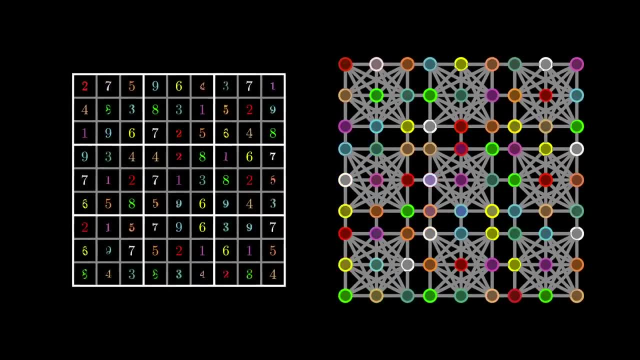 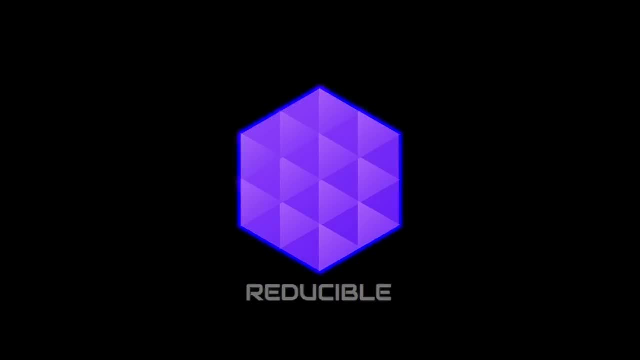 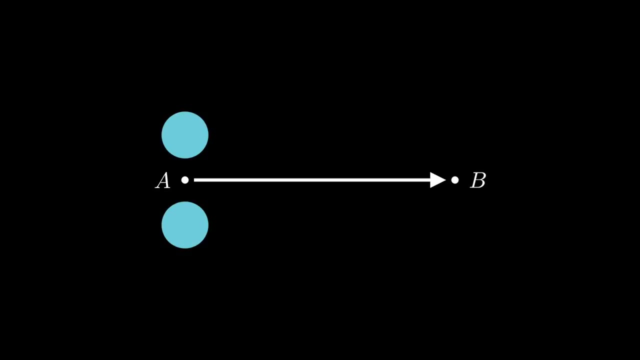 complexity leads to a variety of interesting ideas that show up all over the field of computer graphics. Alright, let's get started. Let's say I want to generate a simple animation that moves a circle. Here's two different animations. One of them looks better than the other. 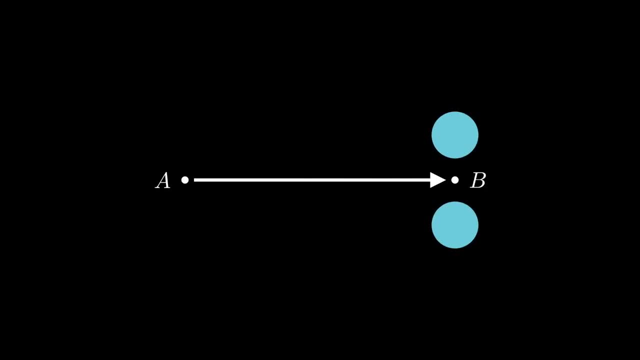 and the reason why is a nice way to introduce how animation works in practice. You see, when you view an animation, you are not actually seeing one fluid motion from point A to point B. What you are really seeing is a sequence of frames In the first animation. 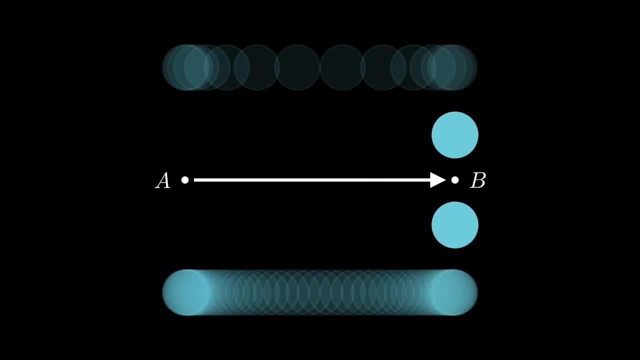 we have 15 frames that are played in one second. Some of you have probably heard of the phrase frames per second or frames per second in computer graphics, but that's not the case. This is the basic idea of frames per second or frame rate used to describe performance of video. 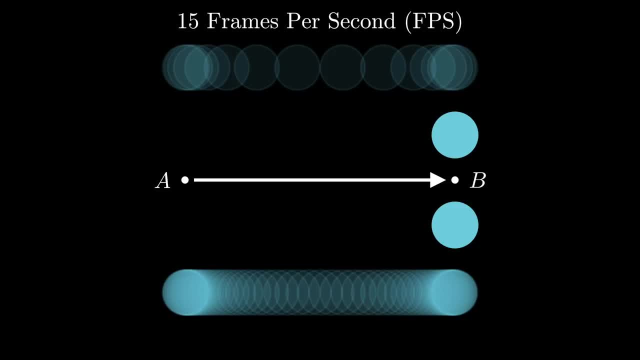 games or cameras, and this is basically what they are talking about. When we unpack the second animation, we have 60 frames played in one second. Because of the higher frame rate, to our eyes, this animation looks significantly more smooth. Now, the main point here is that when generating 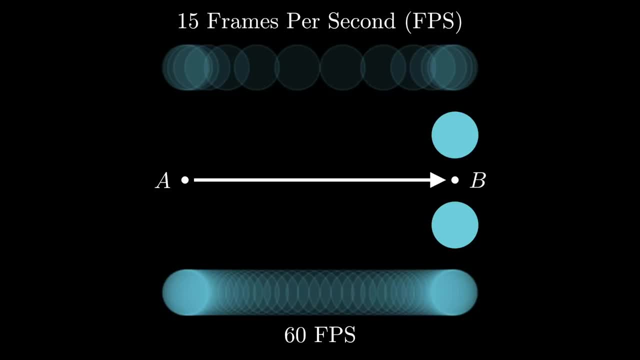 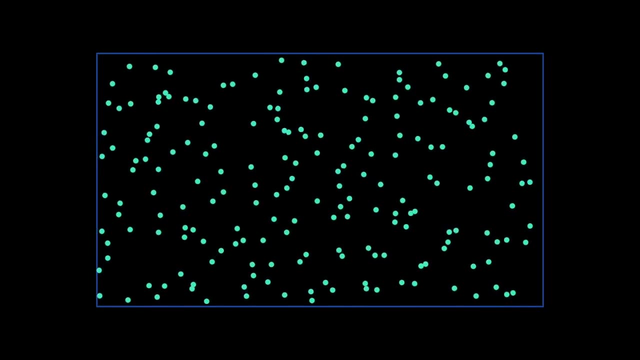 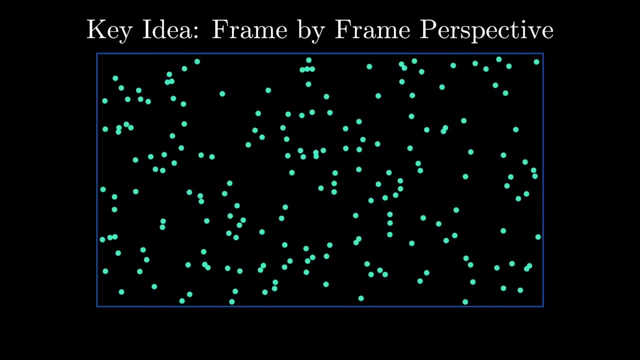 animations or simulations, we have to find some way to create the frames. In this particular example, that's done through interpolation is something we'll touch on later. but in more complex simulations, what we are going to focus on is figuring out how to generate each frame from the initial assumptions of our system. 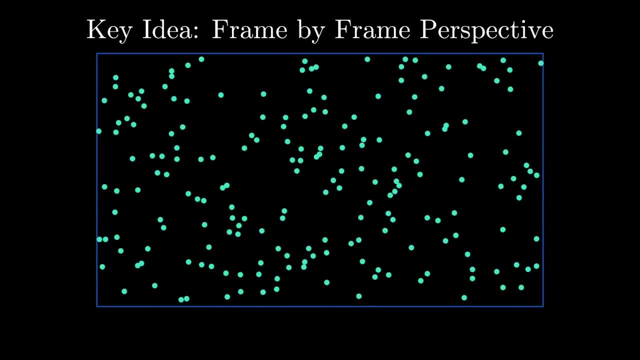 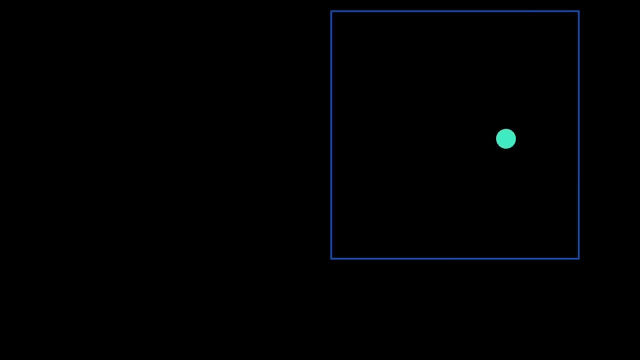 Thinking about animation from this frame by frame perspective makes our life significantly easier. So let's start simple. Here we have a single particle bouncing along the edges of a box. There are three different ideas at play here. The first involves particle dynamics. At every frame, a particle will have a position, velocity and acceleration. To keep things simple, 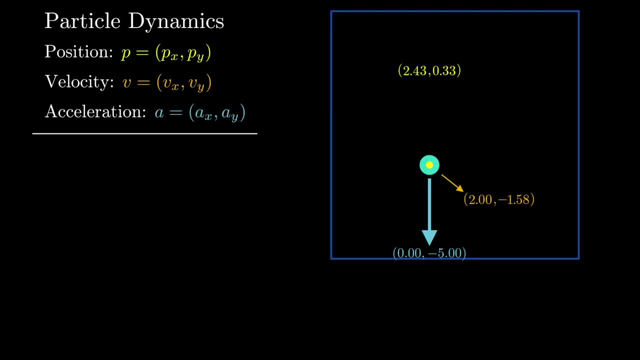 we can enforce the constraint that in all simulations the acceleration will be constant. In most of our simulations later on, in fact, we'll keep this acceleration at zero, but it's worth understanding how to incorporate the acceleration into the dynamics of our simulation. Now, what's nice about the frame by frame perspective that we are taking here is that 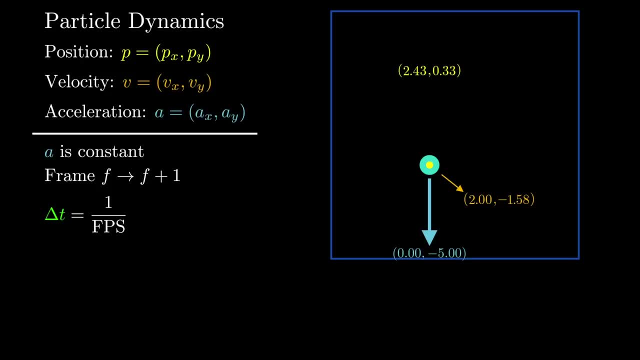 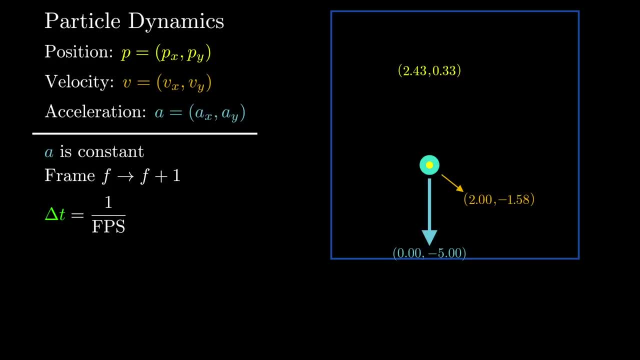 the time between frames is 1 over 60 seconds, Our particle will have some initial position, velocity and acceleration. Given that our acceleration is constant, we get the following updates to our dynamics frame by frame. Here's a quick example of how this plays. 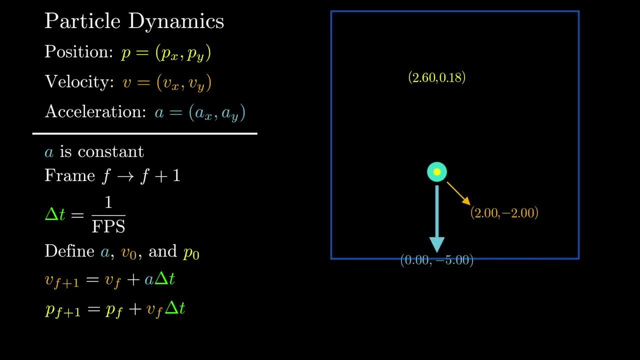 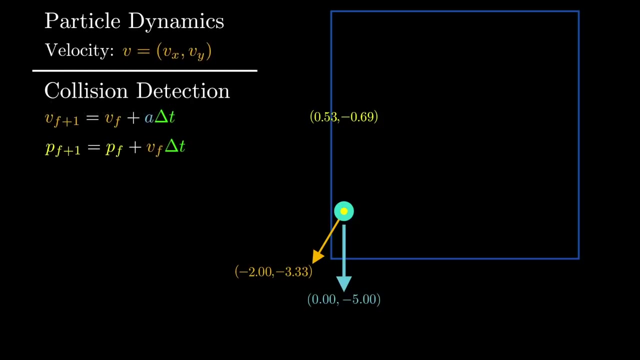 out in a few frames, to make sure this is clear. When you put all the frames together, we have the following: Now, when the particle reaches the edge of this box, that kicks off the second major idea at play: collision detection. This actually turns out to be not too difficult of a problem. 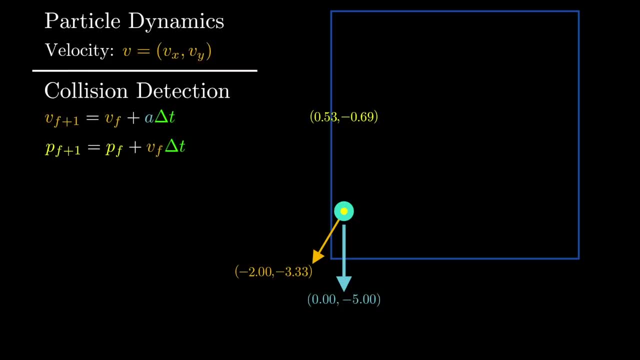 Let's solve it for the left edge. At a particular frame, collision detection between the particle and left edge just requires a comparison between a point and a line. In this case the point is the leftmost point of the circle. If the x coordinate of our point is less than or equal, 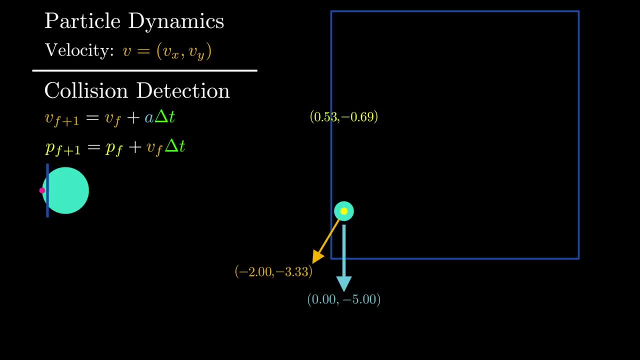 to the x coordinate of the point on the left edge, we have a collision. The logic for all other edges is the same basic principle with slightly different conditions. To show an example in our animation, this is the frame. we actually detect a collision. 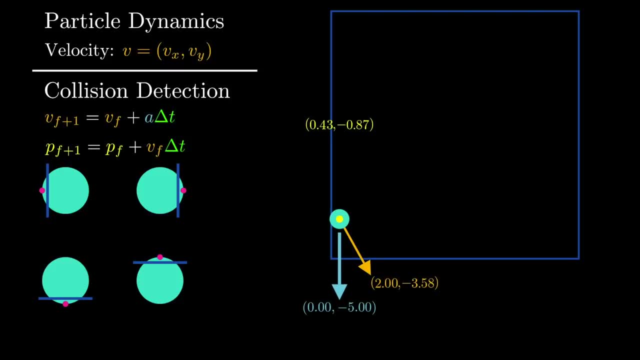 After detecting a collision. the third and final idea involves resolving collisions. Resolving a collision requires updating the dynamics of our colliding objects in a sensible manner, based on the assumptions of our own Collision response can get quite complicated in terms of the math and physics involved. 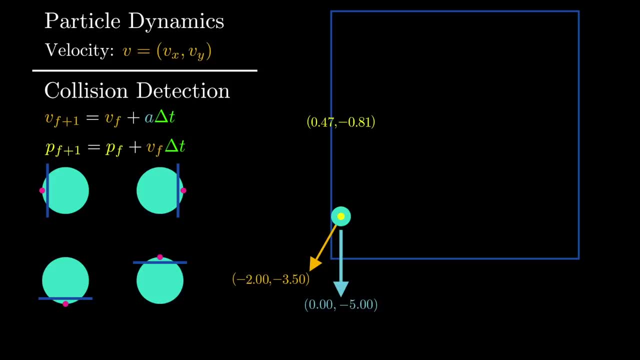 so, to make things simple, we will make an assumption that all collisions between the particle and the wall are totally elastic collisions, so no kinetic energy is lost, and we will treat the walls as having infinite mass. In the case of a collision with the left or the right edges of the box, all this means is the 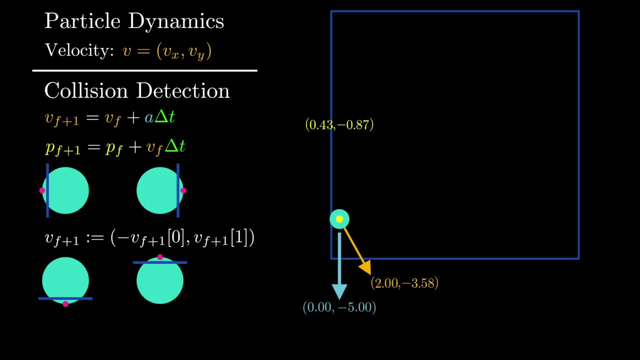 sign of the horizontal component of our velocity is flipped after a collision has been detected. For the top and bottom edges, we flipped the y component of our velocity after detecting a collision. Here are a few more frames to show you what a collision with the bottom edge looks. 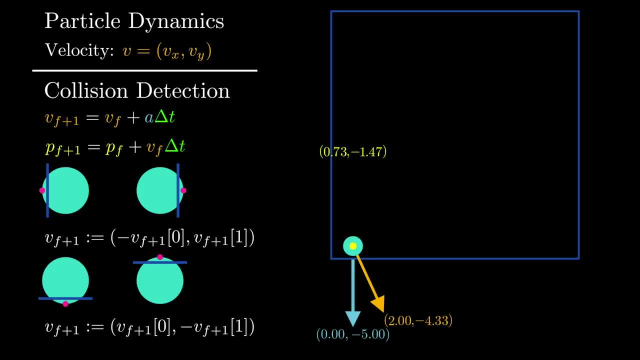 like Notice that the updates to our dynamics, to velocity and position, happen regardless of a collision. Let's put this all together and see what an implementation of this logic looks like. Let's assume we have a particle object that contains information about dynamics. We'll also 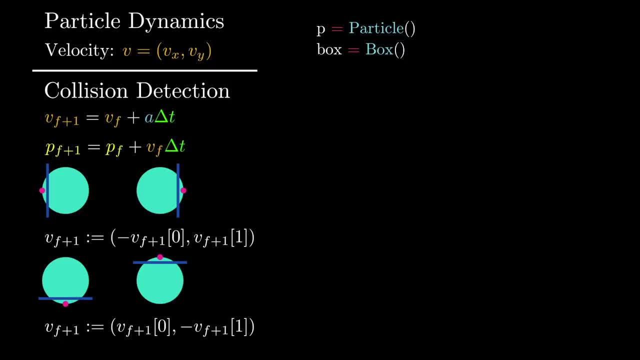 define a function that represents the enclosed space In most animation or game engine frameworks. there's a nice paradigm for updating information frame by frame. How it's usually defined is by an update function, where we are given the time between frames and all we have to do is define how our object's properties change over time. 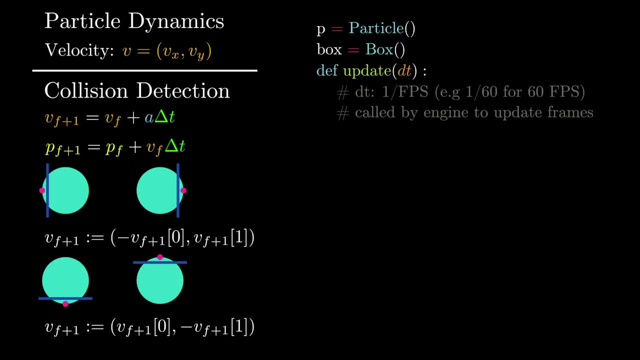 The engine then takes care of calling this function from frame to frame. Given this fact, our update function is actually not too hard to define. We define how the dynamics change from frame to frame, and then we define another function to specifically handle collision detection. Handling collision detection is just a matter of converting the logic we have already. 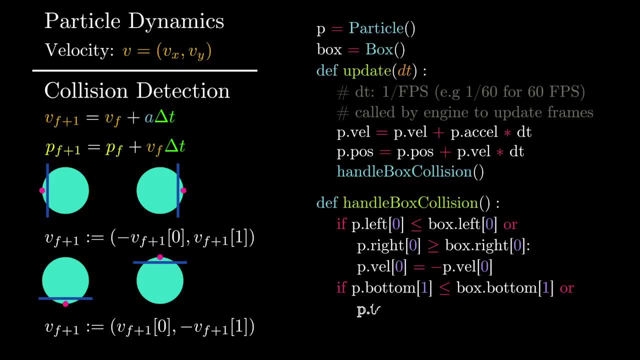 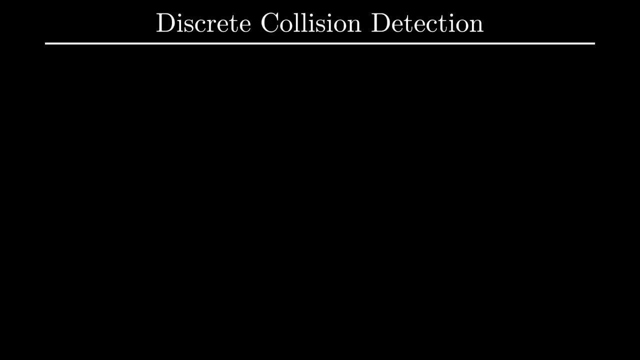 defined into code. Here's what that looks like. So what we just implemented is one example of discrete collision detection. Before we add complexity, it's worth taking some time to address some of the limitations of this framework. Some of you may be thinking what happens if between one frame to another? 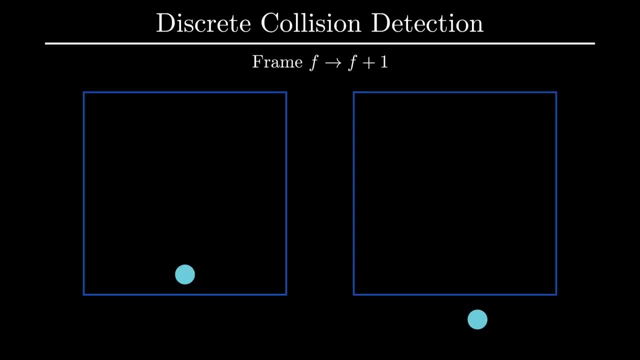 the particle completely passes through an edge. This can happen, especially if the particle is moving quite fast. This issue is so common that it's actually given a name: tunneling. Let me show you an example of tunneling. Yeah, it can be pretty ugly. 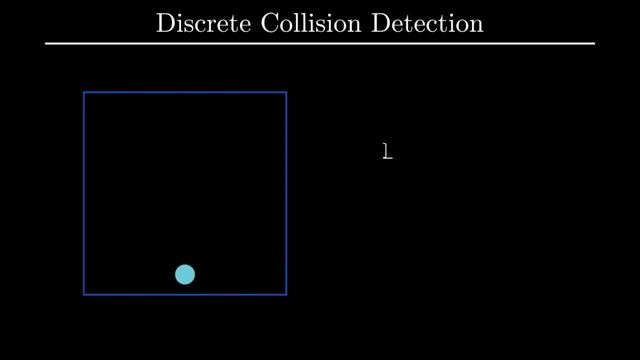 There are two easy solutions to tunneling and one that is substantially more complex. The first easy solution involves making sure particles don't move too fast. Discrete collision detection does have some randomness involved. When particles move slowly, we are more likely to detect collisions and resolve them at an appropriate time. 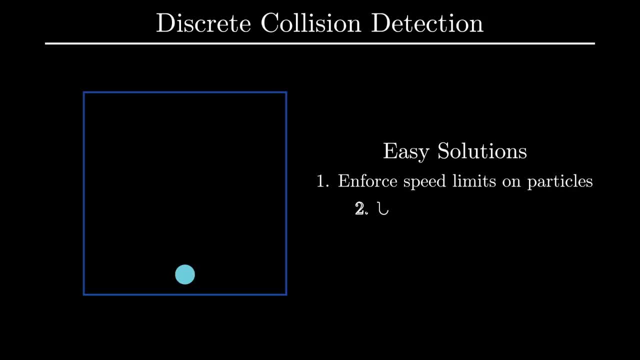 Another solution is a variation of the same idea: Instead of slowing down particles, just take more frames. Both of these solutions work, but obviously they are not ideal and definitely do not work in all cases. The third solution requires taking a bit of a different approach By the nature of discrete collision detection. 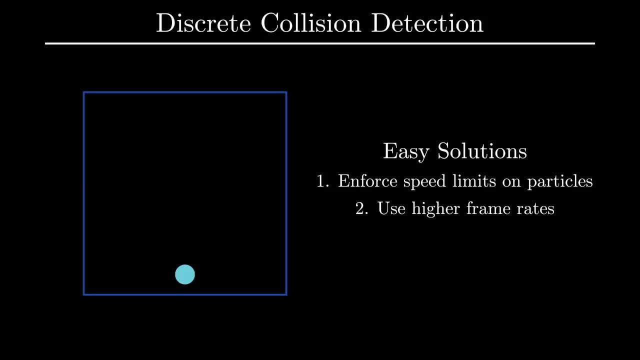 tunneling will always be a possible issue. There's another paradigm in collision detection, called continuous collision detection, that directly attempts to solve this problem. Continuous collision detection is a great showcase for quite a few concepts in computer graphics, so let me give you an overview of how the basic ideas play out. 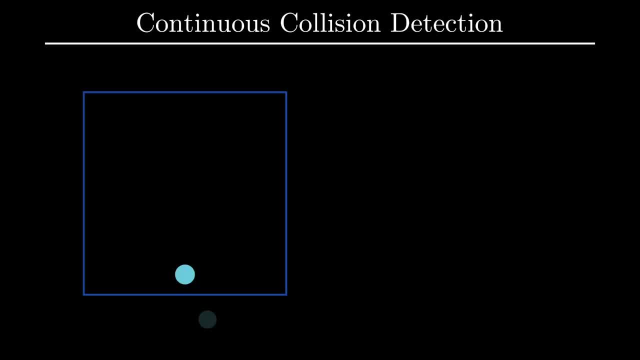 The core problem is that we end up missing our collision because it occurs at some point, and we end up losing our collision because it occurs at some point. So let's label the positions of the particle in these two frames as follows. Frames are played at constant time steps, so let's define the actual coordinates of the. 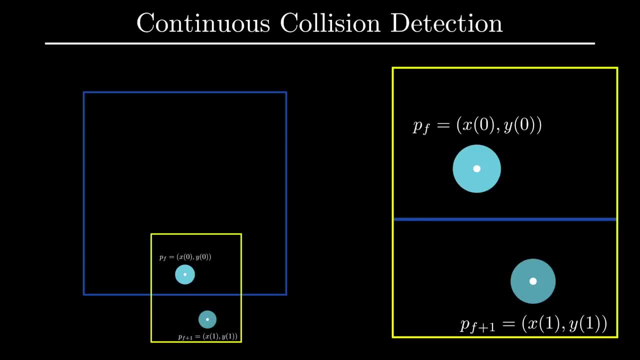 starting and ending point of a particle. in terms of a time, Let the start be at time 0, and the end at time 1.. What I'm basically doing here is I'm parameterizing the x and y coordinates of our particle over time. This is particularly useful, since it allows us to easily define 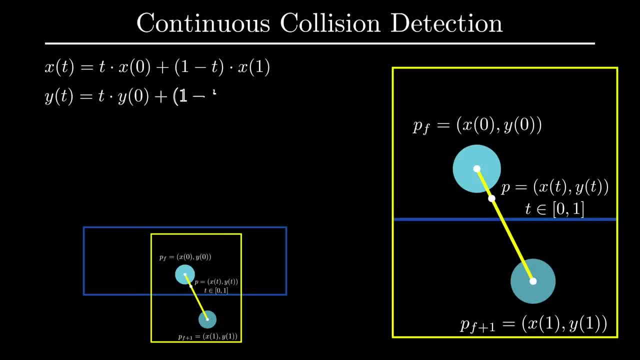 the points of a line given the starting and ending point. This process is called linear interpolation and is actually used all over the place in graphics. An easy way to think about linear interpolation is: it's just the weighted average of the starting and ending points. For example, if t is equal to one half, you get the midpoint. If t is equal. 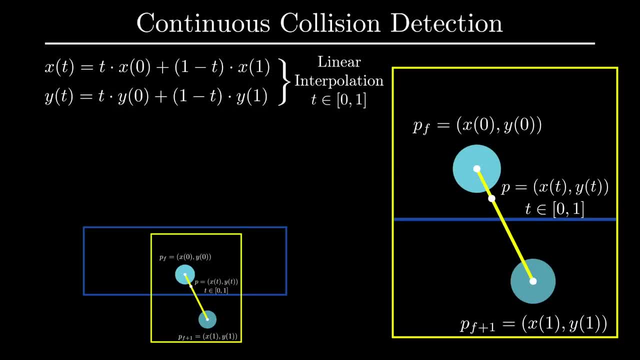 to one fourth, you get a point one quarter of the way along the line from the starting point. The goal of continuous collision detection is to fill out the missing information between frames. What we are really interested in is the exact point of collision, which we can label as follows: 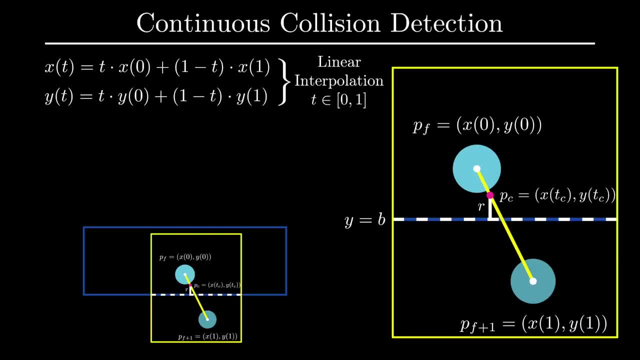 Now, the entire idea behind continuous collision detection is to solve for this point by using the constraints laid out by our collision detection system. In the case of particle collision with a horizontal edge, one constraint is as follows: We know the exact point of collision will occur. 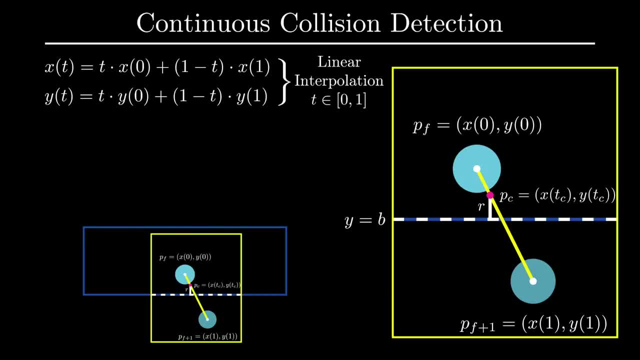 when the center of the particle is distance. So we can find the distance r above the edge of the box, where r is the radius of our particle. This gives us the following relation: We can then combine this constraint with the linear interpolation constraint and get a system of linear equations which we can then solve for. 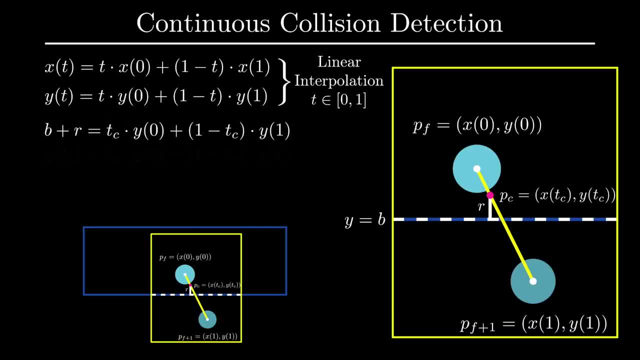 our unknown parameter, tc, or the time of collision. In our particle example, this happens to be about 0.23.. So now that we have the time of collision, continuous collision detection is to figure out the change in trajectory of our object after the collision. In our example, this can be done with some simple geometry. 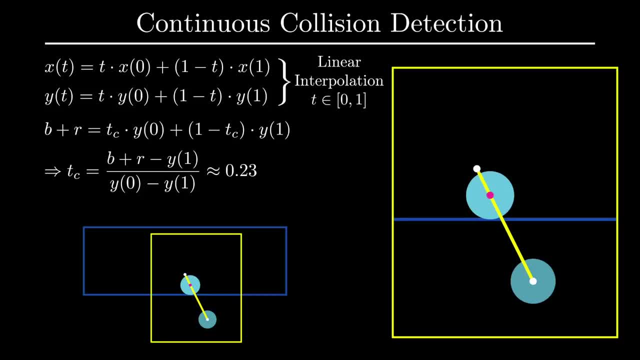 Now that we have the point of collision, the rest of the trajectory is just going to be the original trajectory, flipped over a horizontal line, passing through our point of collision. The reason this works is because we know after a collision, the y component of our velocity will be flipped. 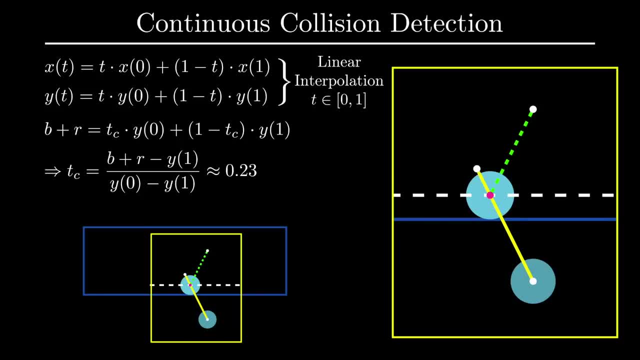 which, geometrically, is equivalent to the y component of our velocity. So we can now get the point of collision, which is a constant. from this point to this reflection, We now have a corrected trajectory of our position, which we can then pass into our 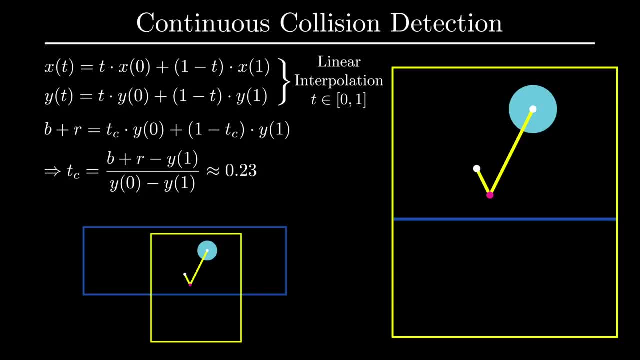 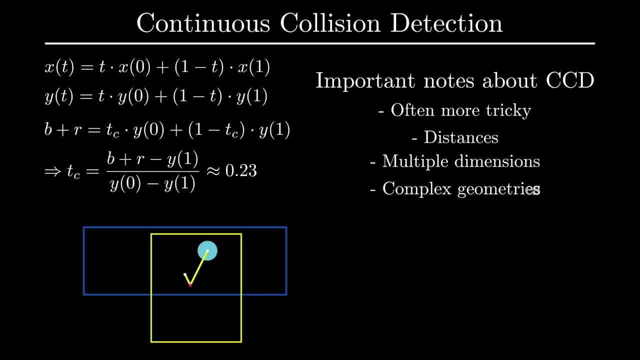 animation engine whenever necessary, and this is a nice solution to tunneling. In practice, however, continuous collision detection can become fairly complex. A lot of times it's not as simple as solving a linear equation. You're often dealing with distances, multiple dimensions and more complicated geometries. 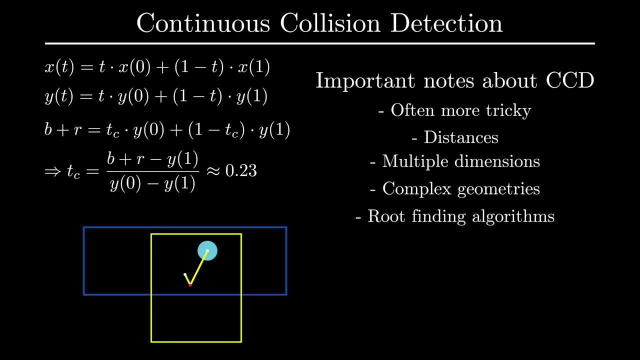 root finding algorithms that can quickly become much more computationally intensive. if you aren't careful, There are entire chapters of books dedicated to this. so there's a lot more I could talk about, but the goal here is to just give you an overview of the basic principles. 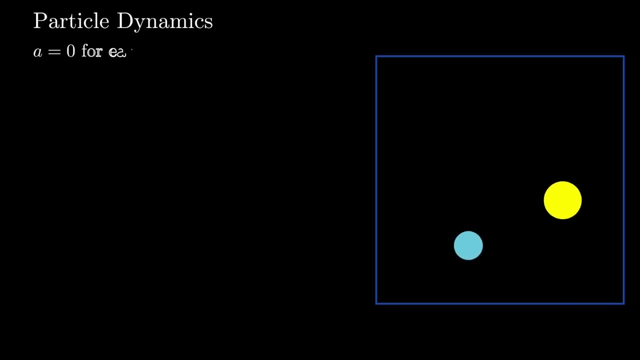 Alright, switching back to the world of discrete collision detection, let's move to a slightly more complex simulation which involves two particles in an enclosed space. Everything from before still applies, but now we have one more feature: particle-particle collision detection and responses. I have some good news and sort of bad news here. 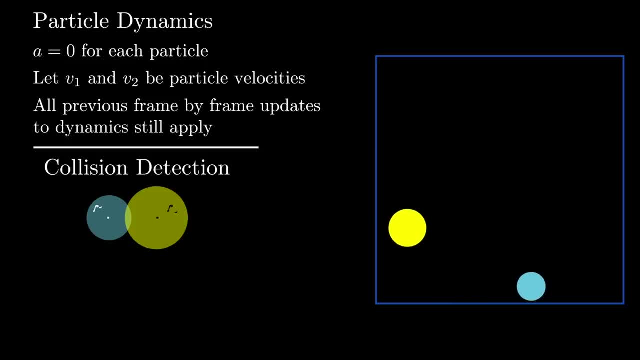 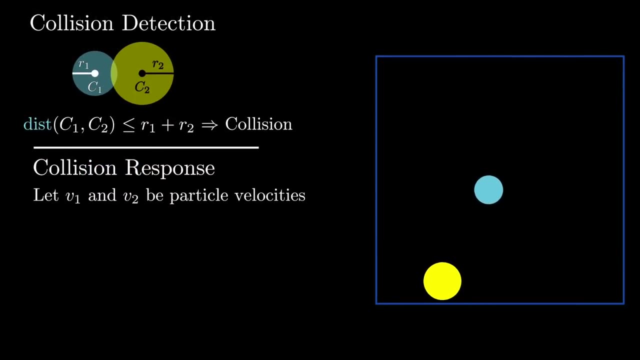 First, the good news: Collision detection between two circles is super easy. All we have to do is check if the distance between the center of the two circles is less than, or equal to, the sum of the two radii. Now the bad news: Collision response is significantly trickier. 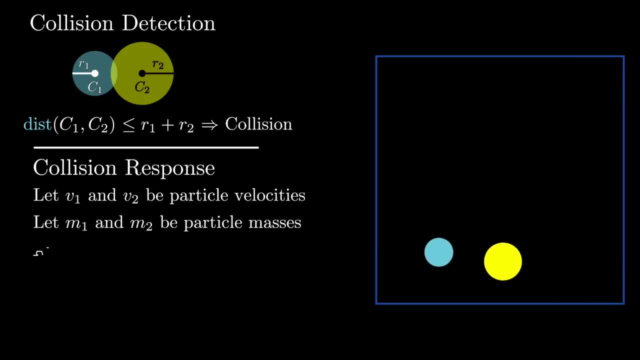 We need to first define particle velocities, Particle masses and then velocities after a collision. To solve collision response for two particles we need to use conservation of momentum and conservation of kinetic energy. I tried working through the equations on my own for two dimensions and long story short. 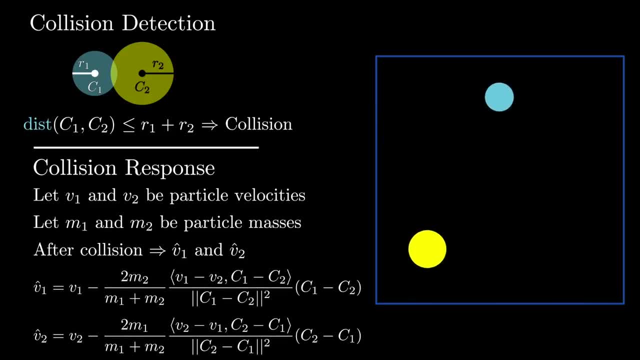 it wasn't fun, So I'm just going to show you the final expressions and I'll leave a link in the description to someone who is way better at deriving and explaining solutions to 2D collisions than I am. I will freely admit that I'm a little bit rusty on my physics. 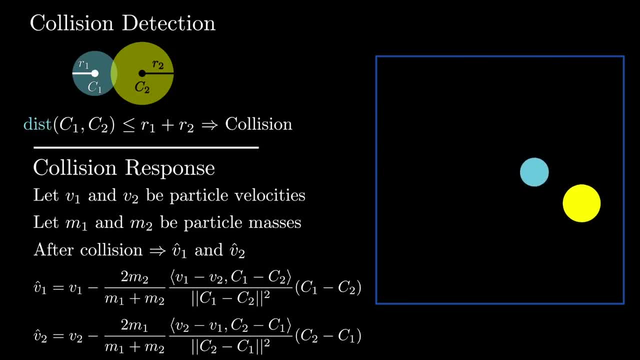 I'm not the best at this. I'm not the best at this. My physics teachers would definitely be disappointed, but I'll live with the shame. So this simulation on the side that I've been casually ignoring is basically created with an implementation of the particle dynamics, collision detection and collision response. 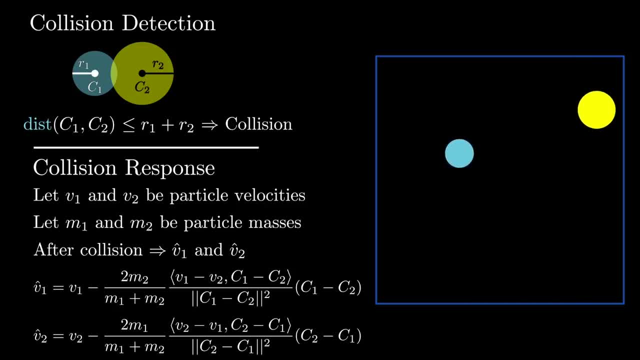 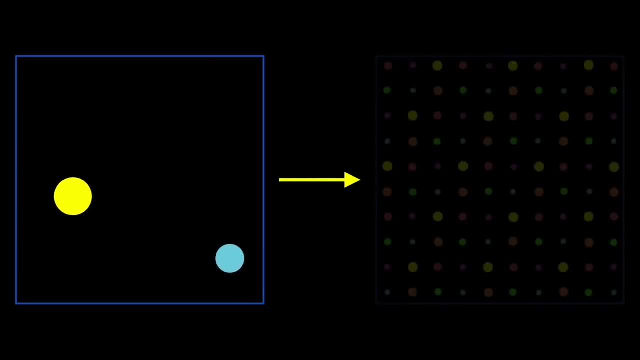 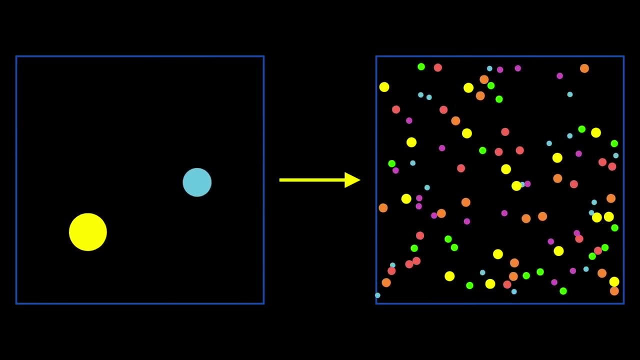 logic we just went through. It actually works quite well, as long as the particles aren't moving ridiculously fast. Now let's add the final and trickiest layer of complexity: Scaling up these simulations. The goal here is to create efficient methods of handling hundreds of particles. 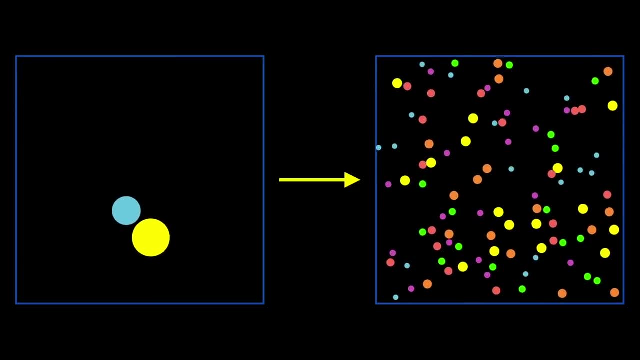 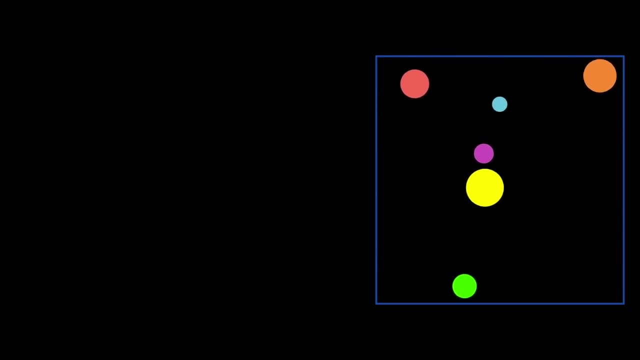 To show the concepts more clearly, though, I'm going to demonstrate the ideas in the context of just six particles. We have a framework to detect and provide responses to collisions between two particles. How do we extend it to multiple particles? Well, the first idea is to just check collisions between every pair of particles. 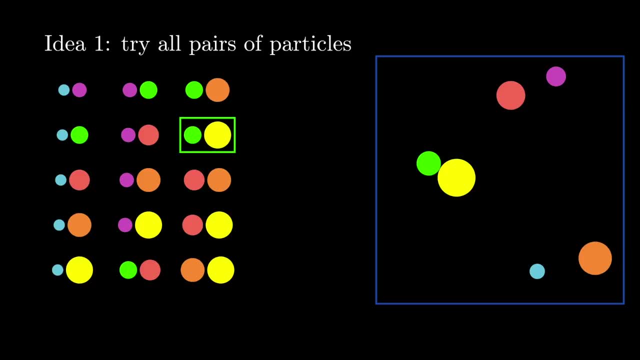 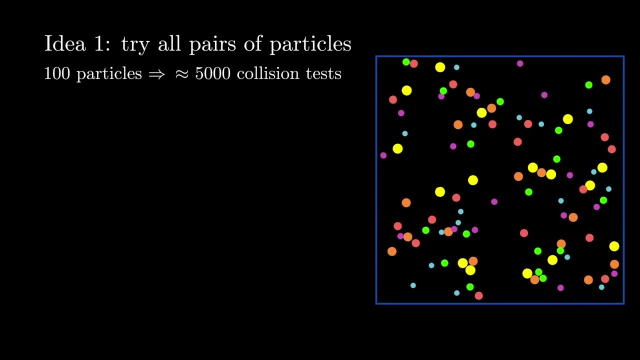 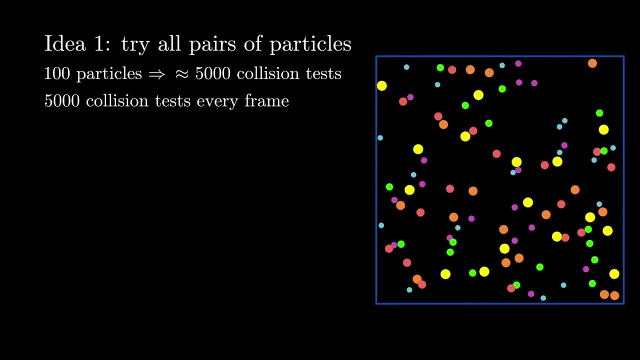 This works, but it gets expensive really fast. For example, on just 100 particles we would have to perform roughly 5000 collisions per second. This doesn't sound too bad, until you realize you have to perform these tests for every single frame in your simulation. 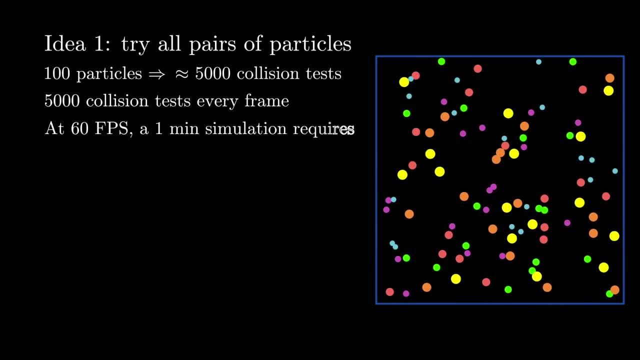 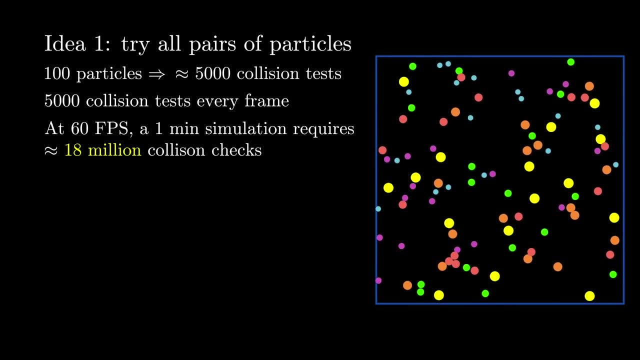 So if you wanted to run a simulation at 60 frames per second for a minute, that would be a total of 3600 frames, leading to roughly 18 million collision tests. I had the awful idea of trying this on my MacBook, just for curiosity and the sounds. 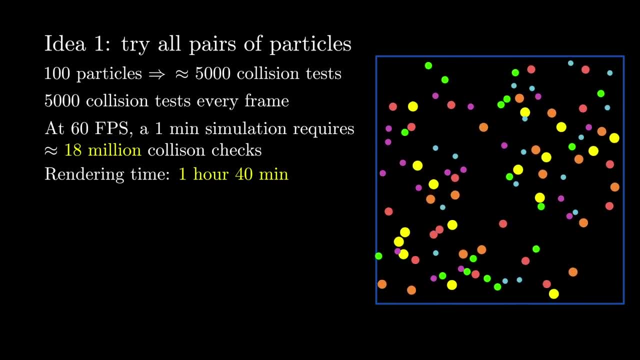 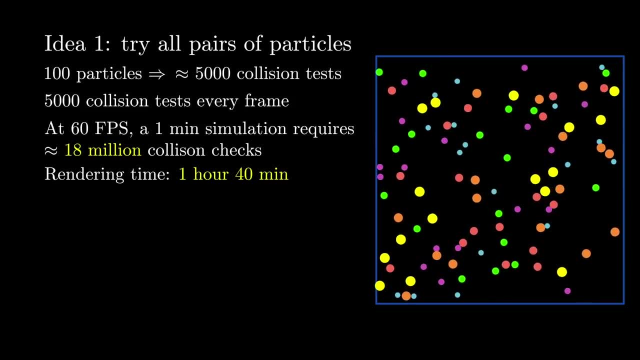 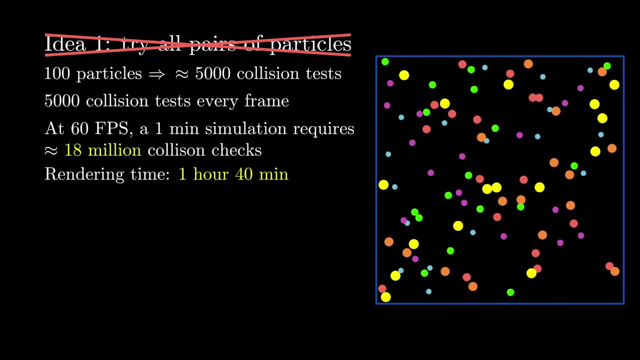 it made throughout the 1 hour and 40 minutes of rendering were quite scary. Don't try this at home And, honestly, you don't even really need these data points to tell you that this naive method of handling collisions among a large number of particles is just an awful algorithm. 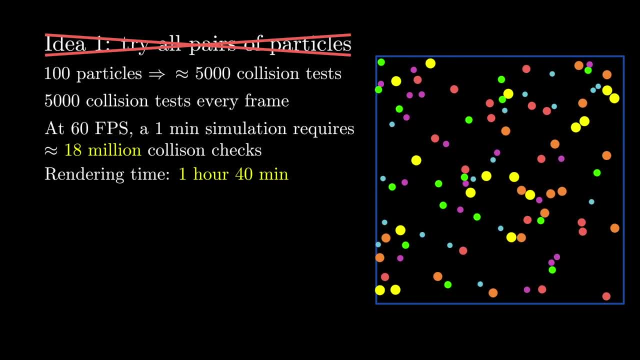 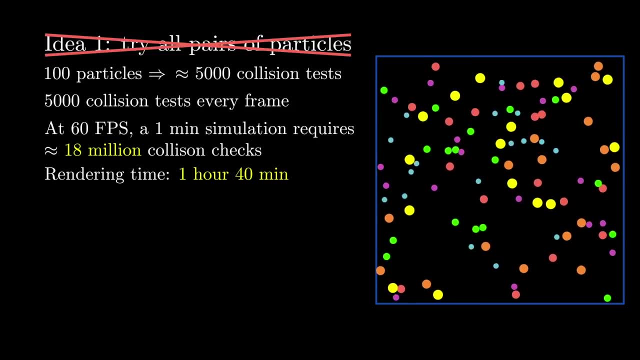 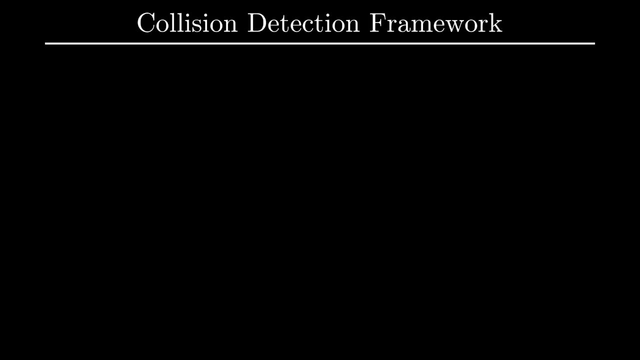 There are so many pairs of particles in this simulation that we would just never even consider testing right. Let's go over a few clever and common optimizations. 1. Solving Collision Detection Problems From a computer graphics perspective. a common framework for thinking about solving collision detection problems at a larger scale is in: 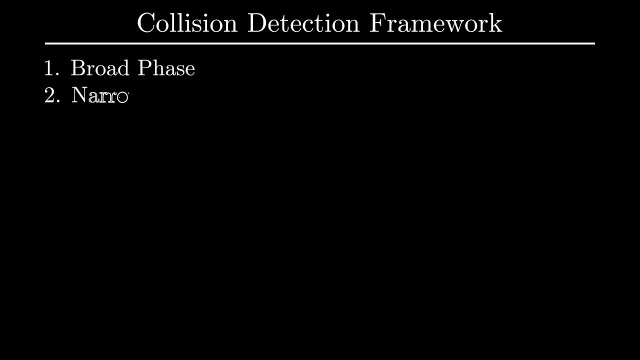 three distinct phases: broad phase, narrow phase- and then actually solving a collision. Broad phase is all about detecting which objects could possibly be colliding, while narrow phase is all about taking the set of possible collisions and finding out what actually collides. 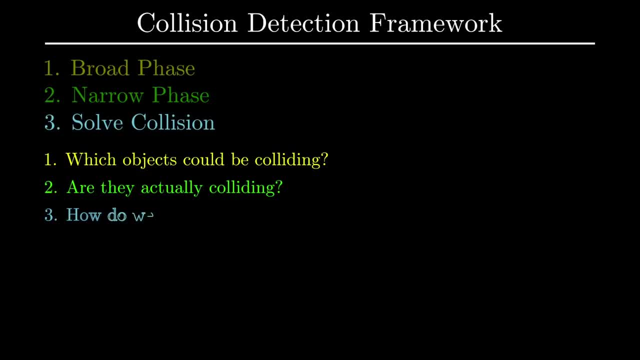 And then solving the collisions. This is all about figuring out the appropriate responses of the objects that did indeed collide. For this particular problem, we've actually already covered the narrow phase and collision response phase. The optimizations that follow are all about the broad phase. 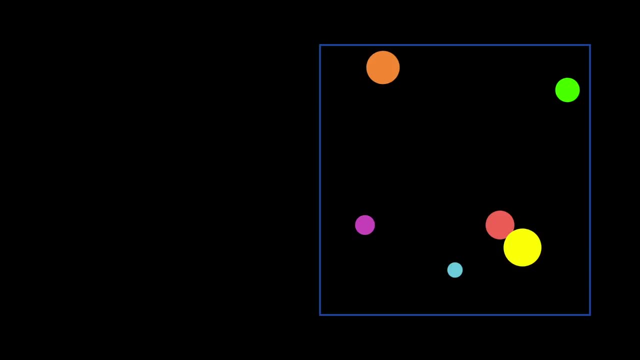 Let's break down these optimizations on a specific frame. These particles all lie on a coordinate plane and one idea of an optimization could be the following: If we take all our particles and project the particles on one axis, this could give us some insight on which particles could be colliding. 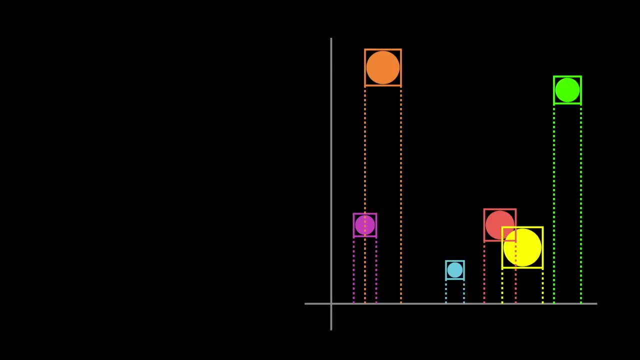 Once we take this projection perspective, we can now simplify particles to intervals, And the idea here is that if there's no intersection between intervals of two particles, there's no way the actual particles will collide. When applied to this particular example, instead of having to check all 15 pairs of particles, 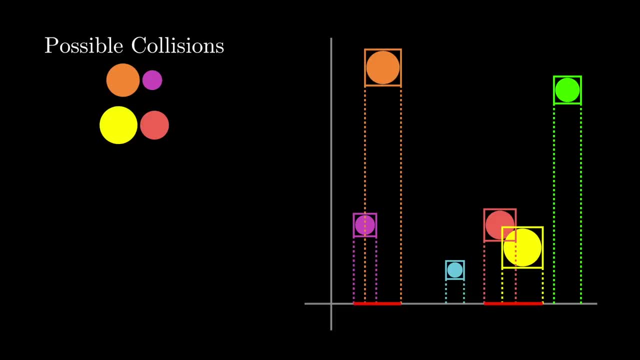 we now narrow down a search to two possible collisions. So let's break down how this algorithm, which is formally called the sweep and prune algorithm, is implemented in practice. The first step involves taking all our particles and sorting it by a particular axis. 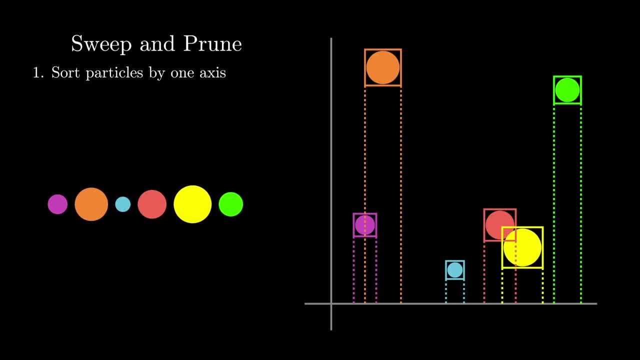 In our example, we chose the x-axis. Now we can think of each particle as an interval on the x-axis. So what we want to do is then maintain a list of active intervals. Initially, The active interval is going to be the first particle in our sorted list. 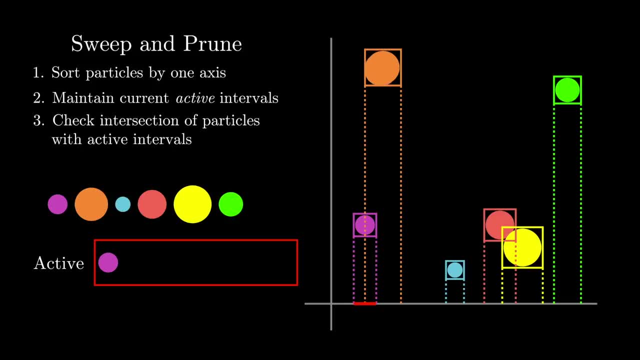 The key idea that makes this algorithm work is that anytime a particle intersects with the current active interval, we have a possible collision. For example, the orange particle's interval along the x-axis intersects with the pink particle's interval, So we report one possible collision. 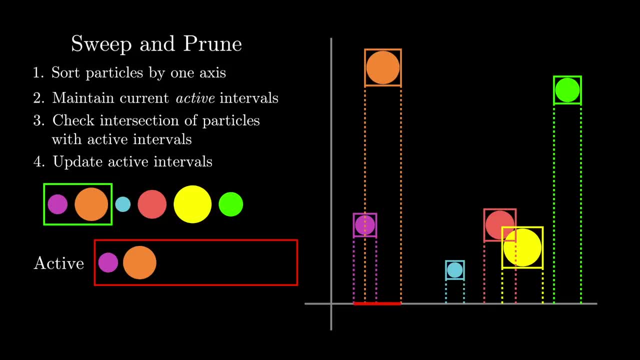 What's also important here is now we update the active interval to include both the pink and orange particles. Another way to think about this is that anytime there are multiple particles in an active interval, we have to check collisions among all pairs of particles. As long as we make sure the active intervals are updated appropriately, this algorithm is 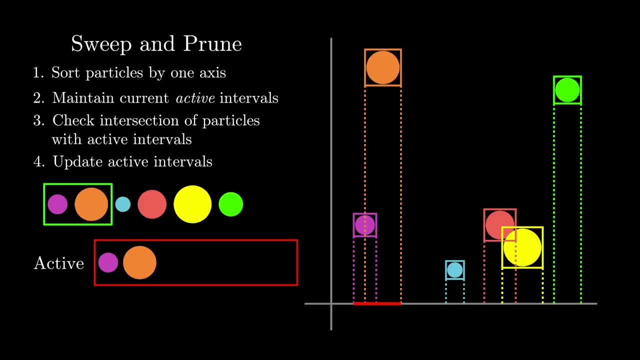 guaranteed to report any particles that actually do collide within its list of possible collisions. The rest of the algorithm proceeds as follows: The next particle in our sorted list is the blue particle, which doesn't actually intersect either of the particles in the active interval. so we now update our active interval to include 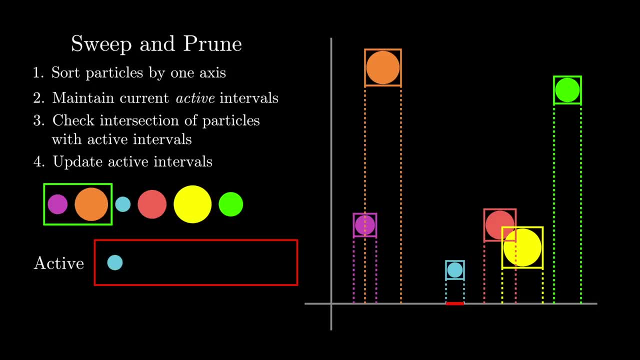 just the blue particle. We then repeat this process on all other particles in our sorted list. There are several further optimizations we can make to this approach, such as performing this simultaneously over multiple axes or picking the axes with the larger variance in particle positions. This can make a difference because there are certain bad inputs. 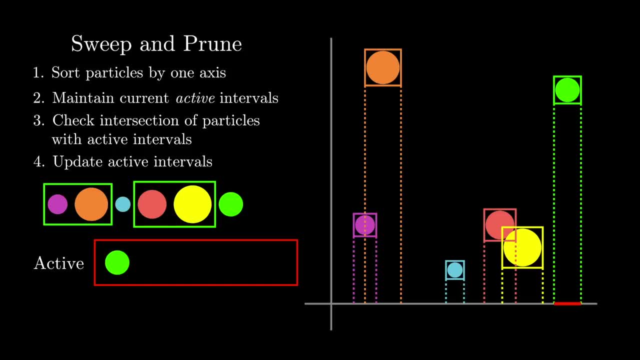 If we pick one axis we don't do much better than a naive scheme. But turns out that in a lot of practical collision detection systems even the simplest version of the sweep and prune approach results in drastic improvements. For example, when I implemented this particular algorithm to render 100 particles at 60 frames, 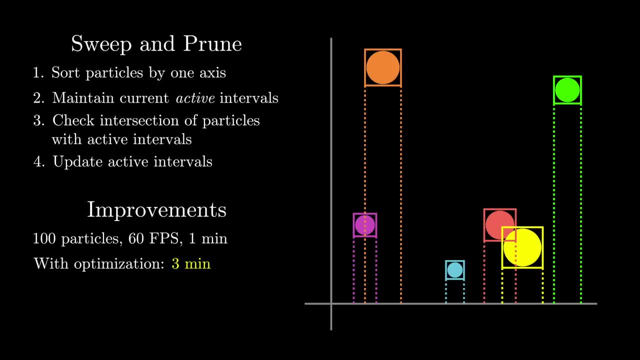 per second for a minute. it only took 3 minutes to render. Yeah, I'm serious. The time reduced from 1 hour and 40 minutes to 3 minutes. That's how much of a difference these optimizations make. So sweep and prune is pretty good for these type of simulations, but there are other options. 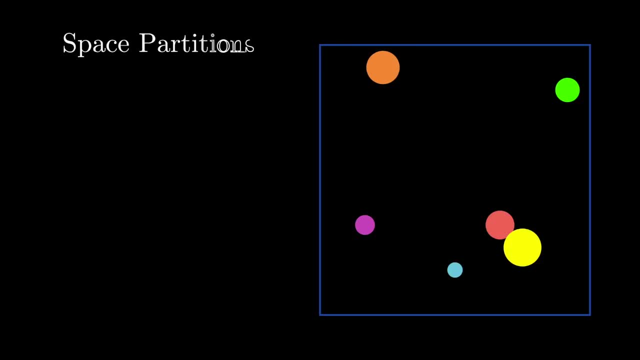 The next big optimization idea involves space partitioning. I want to spend some time on space partitioning, since it shows up in all sorts of applications, not only in graphics, but also in other fields such as machine learning. The simplest space partitioning approach involves uniform grids. 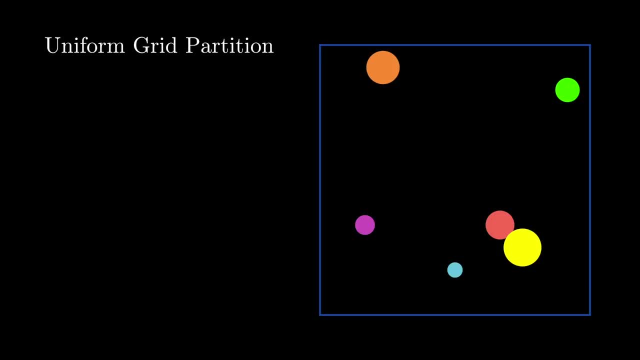 The idea is exactly what you would expect. We split our space into a grid of some length and width. Now what we do is we go through all particles in our simulation and assign them to a cell in our grid. If a particle lies in the intersection of multiple grid cells, we simply keep track. 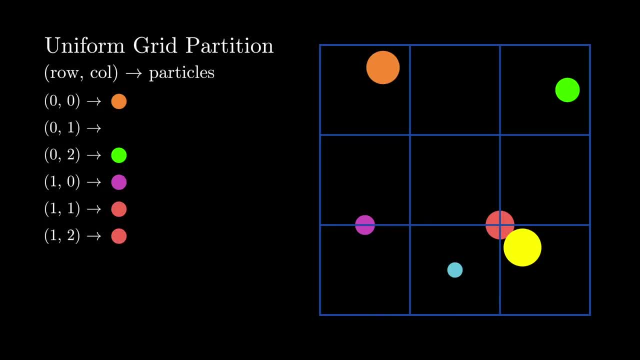 of the particle in all the relevant cells. This is a very simple way to do it. It's a very simple way to do it. Once we have every particle assigned, our set of collisions will only include all pairs of particles within a cell, which will, in practice, give you much better performance. 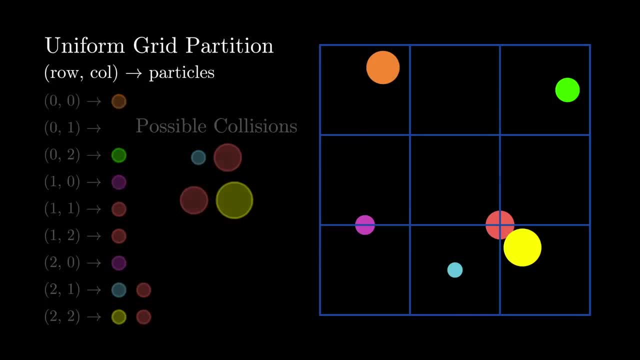 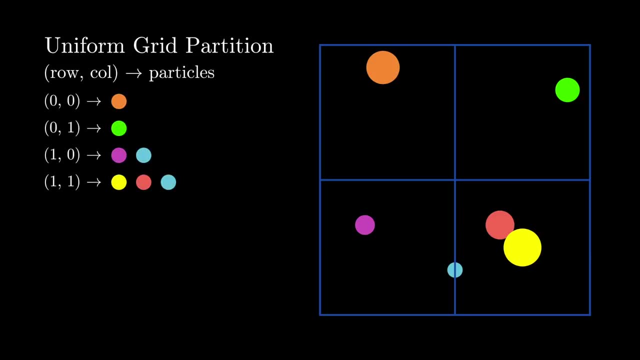 One aspect here that's important is the number of rows and columns we choose as part of our uniform grid strategy. As with most ideas, there is a trade-off: If we have fewer cells, less memory will be used, but more collision checks may be required. 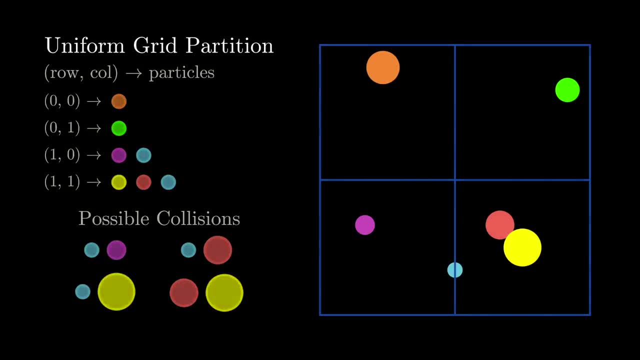 If we have fewer cells, less memory will be used, but more collision checks may be required. If we have fewer cells, less memory will be used, but more collision checks may be required. If we use a larger number of cells, we're more likely to have fewer possible collisions. 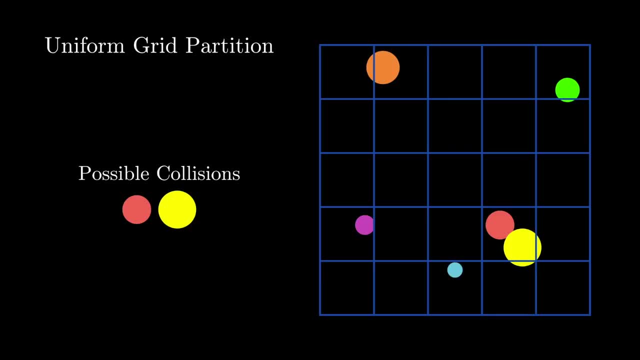 but we will need more memory to store our grid. Another aspect that's a little inefficient about the uniform grid space partitioning approach, especially when there are a lot of cells, is that there could be cases where a large number of the cells are empty and therefore a waste of memory. 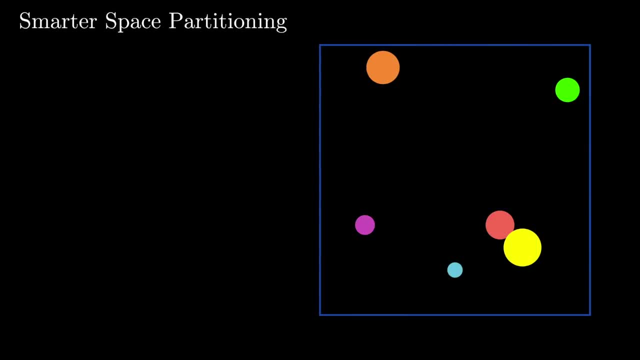 The next type of space partitioning approach tries to utilize the structure of the particles in the scene. to prevent this issue, Let me introduce you to KD trees. Instead of uniformly splitting the space, let's pick an axis and split the space by the median. 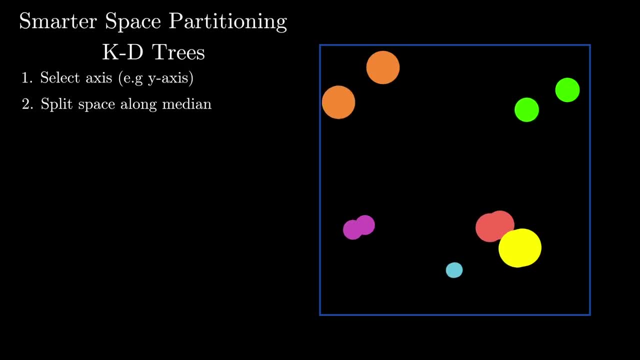 So, for example, here we chose the y-axis, and if we sort objects along the y-axis, the median passes through the pink and red particles. We now have split the space into two subspaces, and the key idea behind KD trees is: we're. 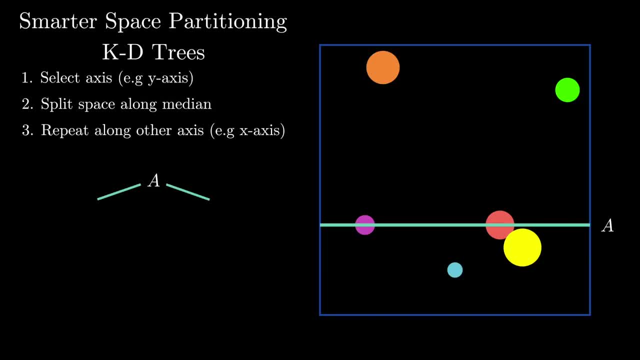 going to do the same process on each of these subspaces on the opposite axis. So since we initially picked the y-axis, we're going to split out two subspaces along the median of the x-axis. On the bottom subspace we have four objects. 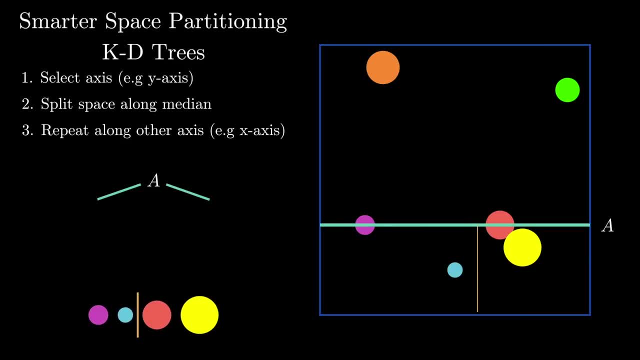 If we sort them along the x-axis and find the median, we get the following split. We repeat the process on the top subspace. Now notice what we have done: With just three splits. We've balanced out the two subspaces. We've sorted out the objects in each space. 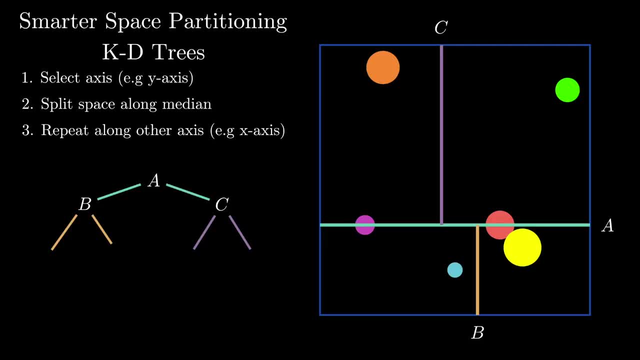 In other words, every space is being used to store objects, which may be advantageous if we don't want to waste any memory. This type of split also naturally gives us a tree structure, and trees tend to be more efficient to traverse than grid-like data structures. 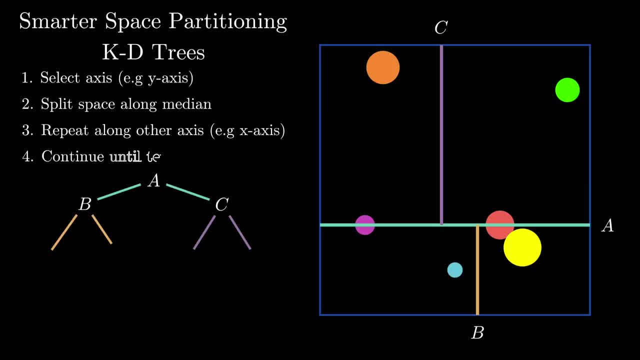 Now we could stop here, but usually with KD trees we generally have some termination condition. The termination conditions can be a variety of things: Some simple, such as the limit on the number of splits or the number of particles in a partition of the space. 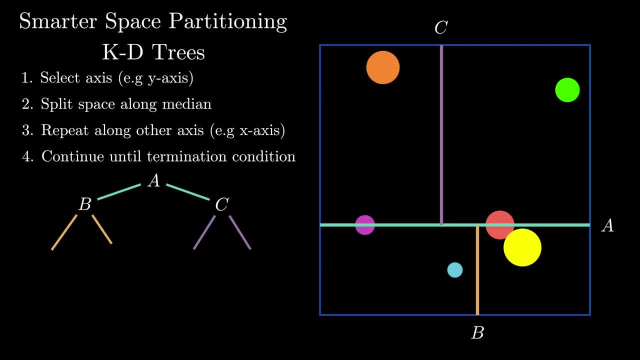 Some more advanced techniques also exist, where we basically continue splitting until we can no longer partition the space in a way that is advantageous. Here let me show you an example of what this means. We can add one more split to the upper left space, since that will give the two new spaces. 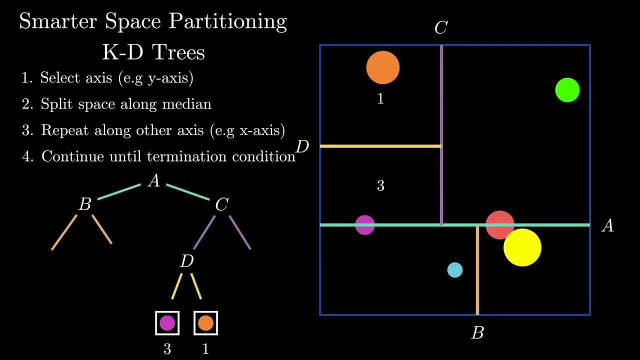 only one particle. Spaces with one particle are really nice, since we don't have to worry about any collisions in those partitions. We can do the same split on the upper right and lower left spaces, giving us the same tree. The bottom right space, however, is a special case, since any potential split along the median 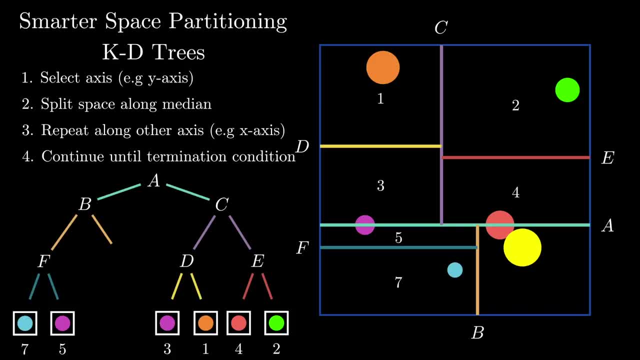 of the two particles will not be beneficial, since both spaces will still have two particles. So in this case, it makes sense for this space to no longer be divided, making this our final tree structure. When figuring out which particles could potentially collide, all we have to do is traverse the 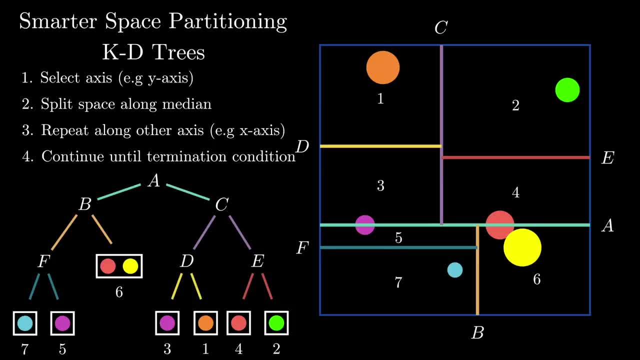 tree and get the leaves of the tree. For any leaves that have more than one particle, we include all pairs into the set of possible collisions. In this case, there's only one possible collision, which happens to be the only collision in our example. 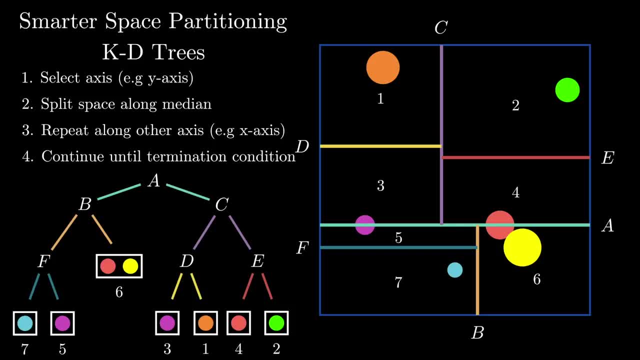 The final scheme I want to show you takes a slightly different approach. Sometimes it's really annoying to have objects in multiple spaces. This is especially true if the object in our collision detection schemes are complex geometries, where performing collision checks is a must. In this case, space partitioning schemes can actually be quite awful. 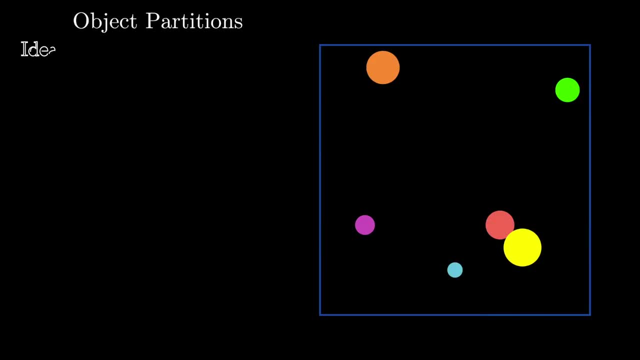 So another idea is to use an object partitioning approach where the key idea requires that we never allow objects to overlap spaces. The most common object partitioning method that shows up in a ton of computer graphics applications is bounding volume hierarchies. These data structures are so important in graphics that there are entire chapters of 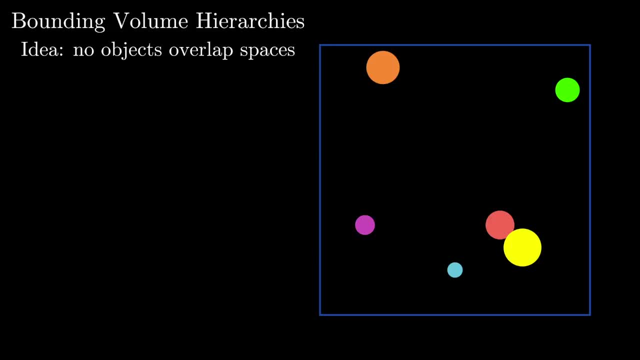 books dedicated to them, But I'll give you some insight into the basic ideas of how these work. There are many methods for constructing bounding volume hierarchies, but one of the most common ways to do it is as follows: We first pick an axis and then pick the median object along the axis. 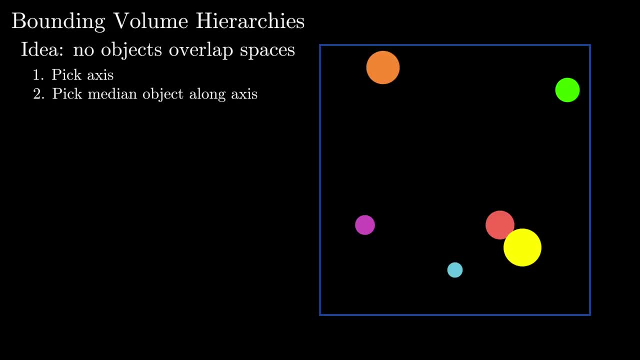 This is a little bit different from the KD tree, because we are now going to use this median object to split our initial set of objects into two distinct subsets. Here let me show you what I mean. If we use the x-axis, there is no single median object. 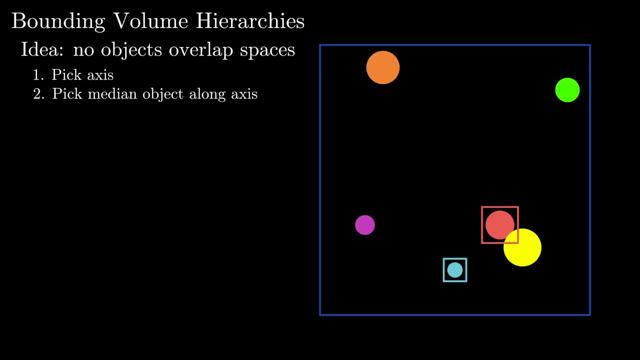 We end up having to choose between the following two objects. So what we do is we assign everything to the left of the blue particle to a set and everything to the right of the red particle to another distinct set. We now define a tight bounding box to encompass the objects of both these sets. 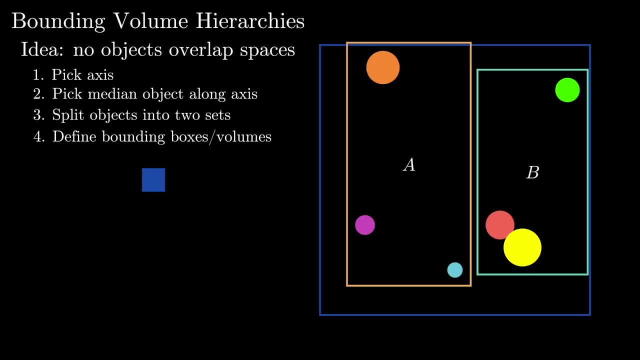 Now, what have we done here? We have now split our space into two subspaces, But the key advantage to this scheme is: no object will overlap two spaces, But of course this is at the expense that spaces could potentially overlap, so as with 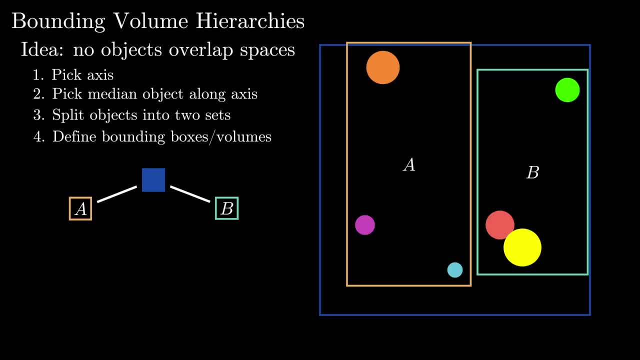 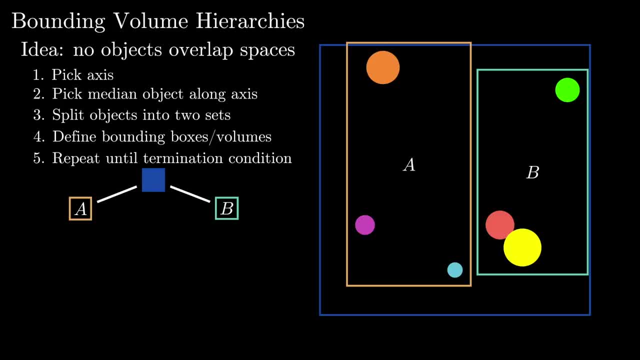 same. let's continue until we get to one object in each bounding box, Starting with bounding box A. let's pick the y-axis and split among the median of the three enclosed objects. The median in this case is a singular object which we can assign. 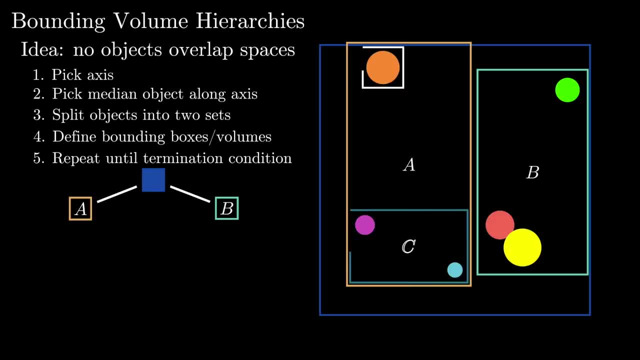 arbitrarily to be part of the bottom left bounding box C, leaving the orange particle to be the only particle in the upper left bounding box. We can repeat a similar process for bounding box B. Continuing on to bounding box C, we can further split it into singular sets of particles and 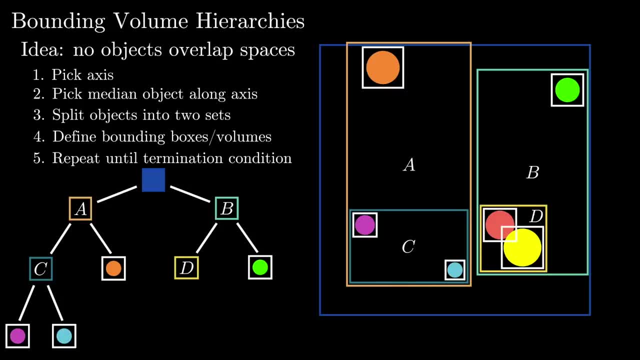 we can do the exact same thing with bounding volume D. Now notice that the bounding volumes that contain the red and yellow particles intersect, and that's the key idea behind finding possible collisions. If bounding volumes don't intersect, there is no way objects. 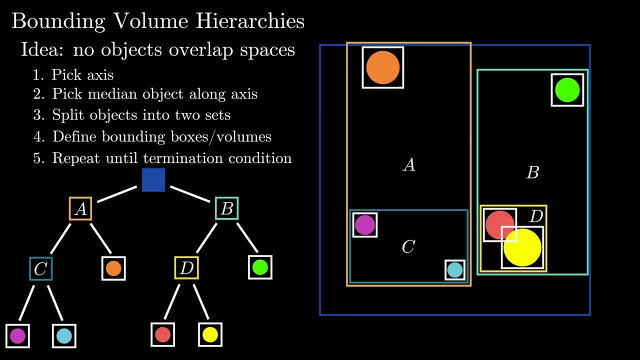 in them will ever collide, which eliminates a significant amount of bounding volume. The algorithm for finding possible collisions is a little bit more involved than spatial partitions, but the core idea involves traversing the tree and checking for intersections between the bounding volumes that encompass the nodes. 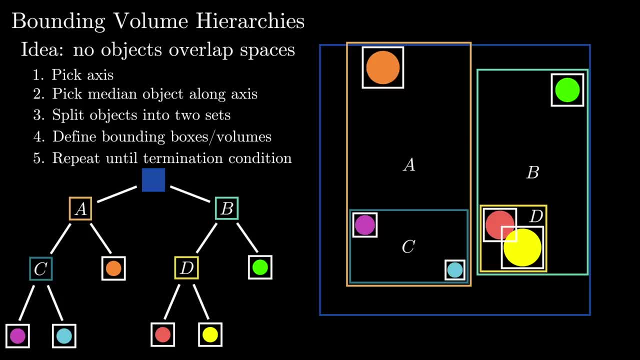 I'll add a few resources in the description that go through this algorithm in more detail for those of you that are interested. Like I said, there are entire chapters of books that focus on this topic, so this is really meant to be an intro to the big ideas. So